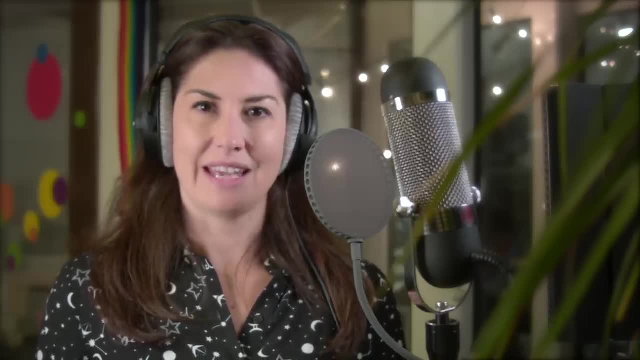 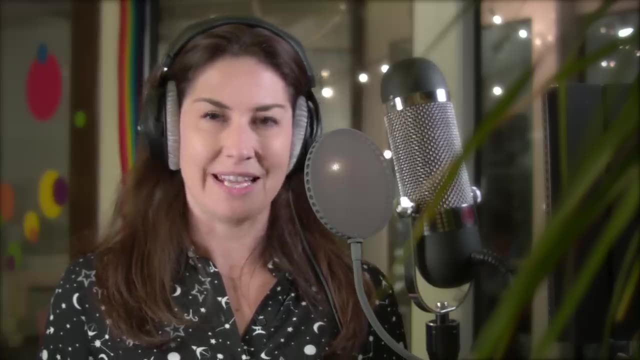 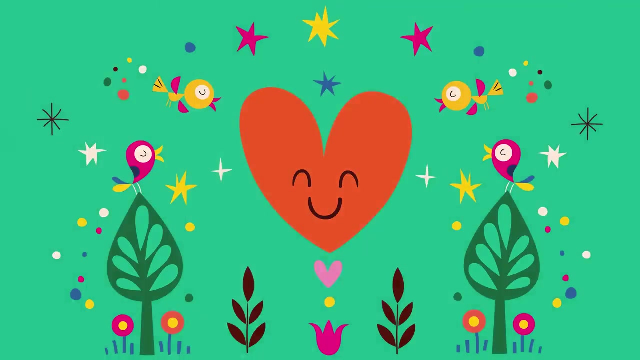 In and out. Next time, as you breathe out, let your eyes softly close, if they aren't already. Now you can allow your mind to make the pictures like a dream. You're standing by a big lake And all around it are trees and mountains. It's beautiful. You look at the water and 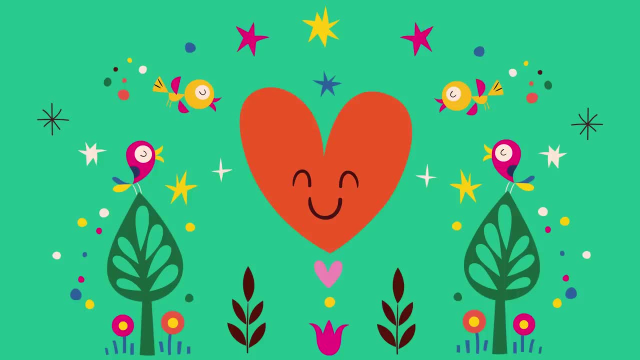 see it's totally still No breeze, no ripples. It looks like glass, Calm, still water. It's peaceful. here In your pocket you have collected some pebbles. You reach inside your pocket and hold one in your hand. It's smooth, cold and round. You take it out of your pocket and hold the. 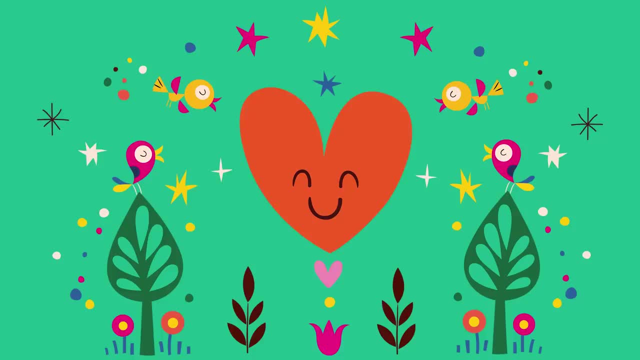 pebble out in front of you over the lake, And you make a special, friendly wish, A wish for yourself: May I be happy, May I be safe, May I be well. You drop the pebble into the water, The ripples. 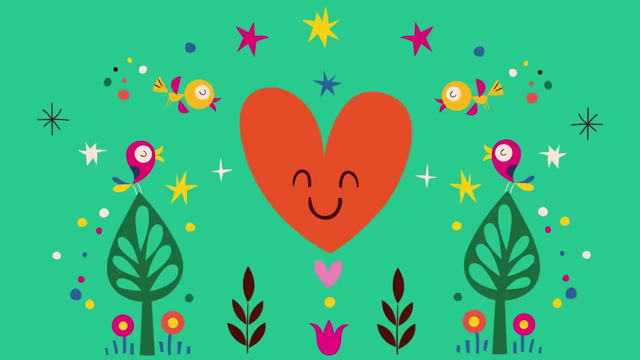 spread. Your wish has landed, You reach back into your pocket for another pebble, taking it out again and holding it over the water. This time you think of someone you like very much, a friend, a family member, someone who makes you happy. As you think of them, you send them your friendly. 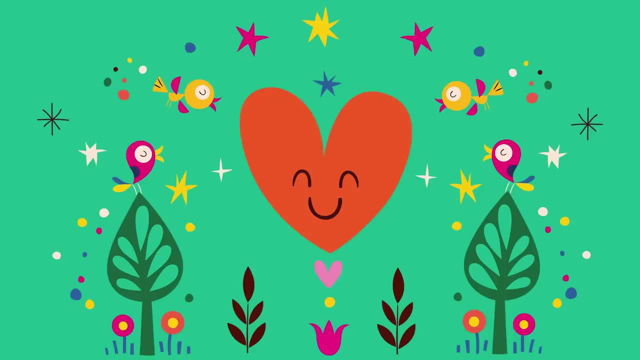 wish. May you be happy, May you be safe, May you be well. You drop the pebble into the water, The wish spreading through the ripples where it landed, passing through the calm water, You reach again for another pebble, holding it in front of you over the water. Now you think of someone. you 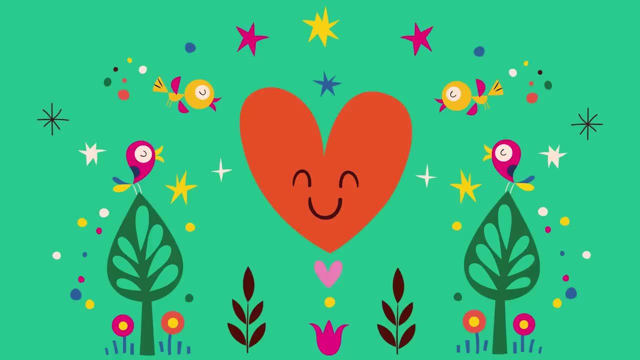 know, You're familiar with them, but you don't have strong feelings about them. You don't have anything that you think of them. This time you're thinking of someone you know, A friend, someone you know a neighbor, a shopkeeper or someone you might see in the street. Think of them and send. 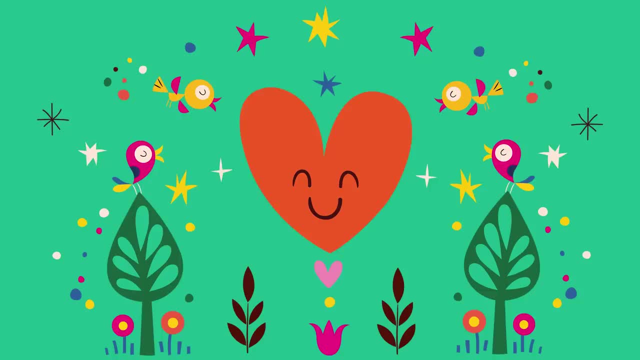 them a friendly wish. May you be happy, May you be safe, May you be well. You drop the pebble into the water. The ripples spread again. Your wish has landed. Your wish has landed You're and your wish lands. 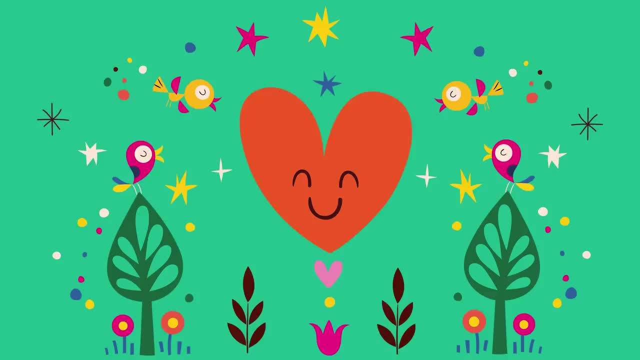 You reach back into your pocket and find one final pebble, taking it out, holding it over the water. Now think of someone you don't like very much. You're not so fond of them, Someone who upset you or you don't get on with. 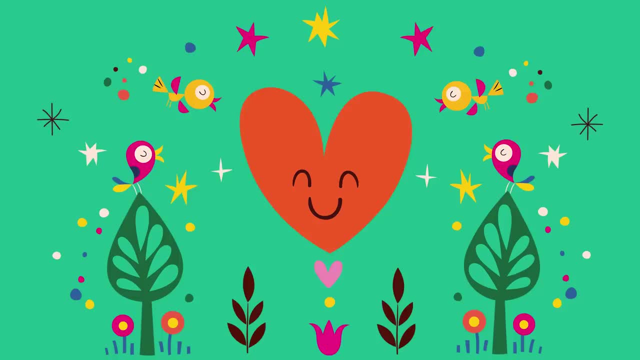 See if you can imagine them now in your mind. You do something amazing. You send a friendly wish to them. May you be happy, May you be safe, May you be well Dropping the pebble. your peace and friendly wishes spread. 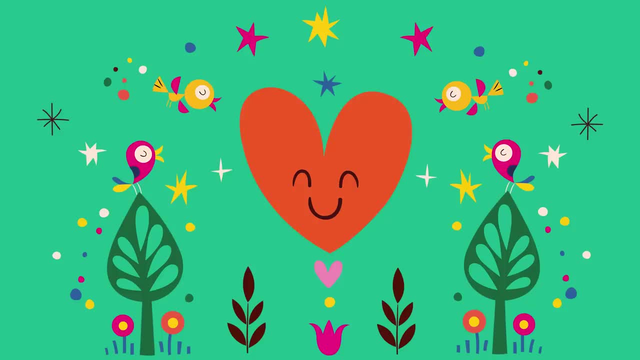 Like ripples on the water. We imagine the whole world and everyone in it, sending our friendly wishes to all. May we all be happy, May we all be safe. May we all be well. Your friendly wishes will make the world a better place.